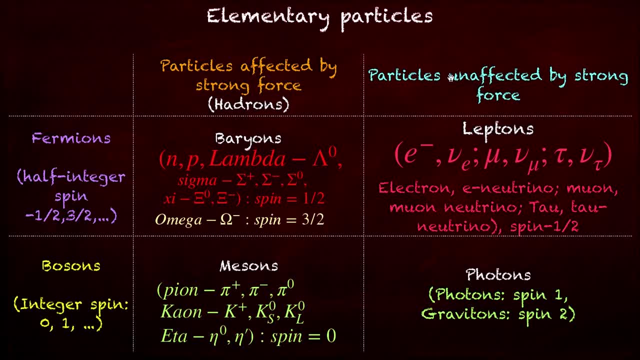 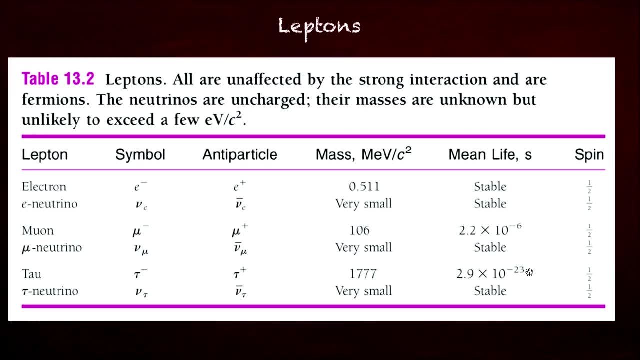 Hadrons contains baryons as well as mesons And particles unaffected by strong force are the leptons and the photons. Now we know the leptons in details. There are electron, electron neutrino, muon, muon neutrino, tau particle and tau neutrino. All of these are fermionic particles. 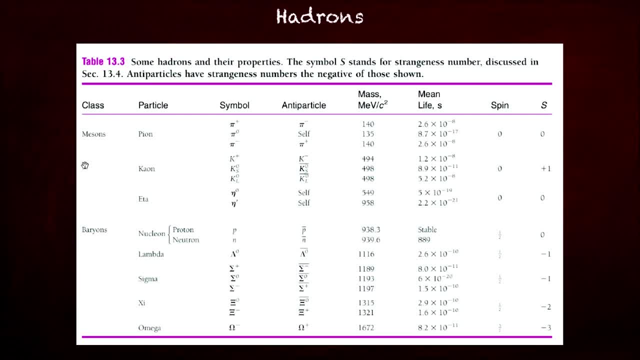 Now, in the hadrons we have baryons as well as mesons. Baryons consist of nucleotides, baryons as well as hyperons, such as lambda, sigma, psi and omega. particle Mesons consist of pi mesons, k mesons and eta mesons. Now, apart from these listed elementary particles, 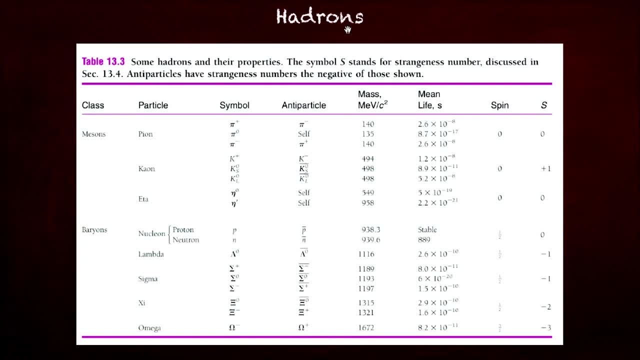 such as leptons and hadrons we discussed. there are many other elementary particles, like resonant particles, which are ultra short lived. So in this we have discussed the leptons and hadrons. So in this we have discussed the leptons and hadrons. 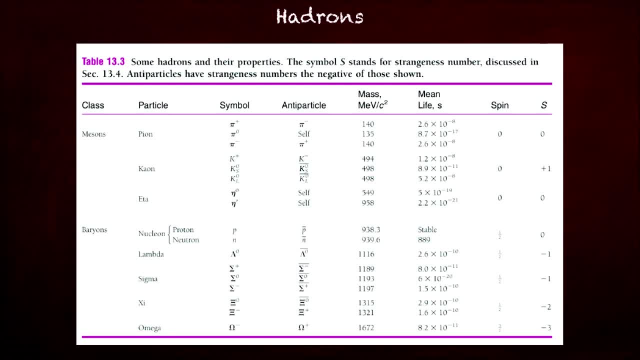 So in this we have discussed the leptons and hadrons. Now many others are also told that there are. according to ourchéries, there might be someルmes, And rest of them we've discussed. So I'm going to fight with these. 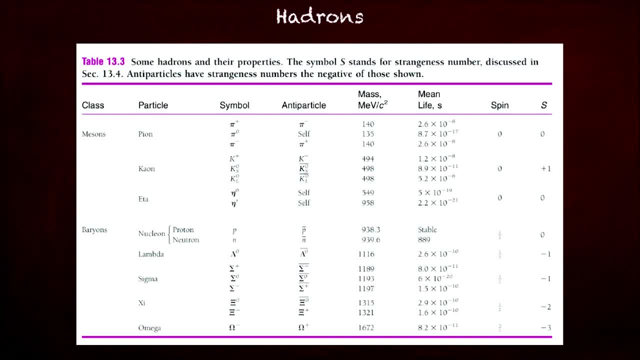 People. now someone is giving you sentences to helpful newspaper articles, Fool etc. they just wrote: okay, decay and any decomposition transformation occur older than to become another very difficult I to the process on okay for other when data- I'm a little particle for the quantum number ascended down for the ordering your reaction day. 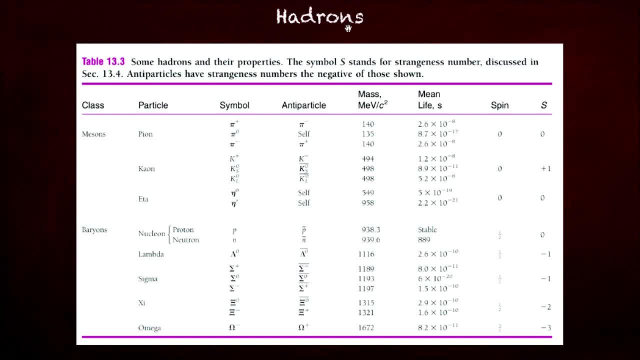 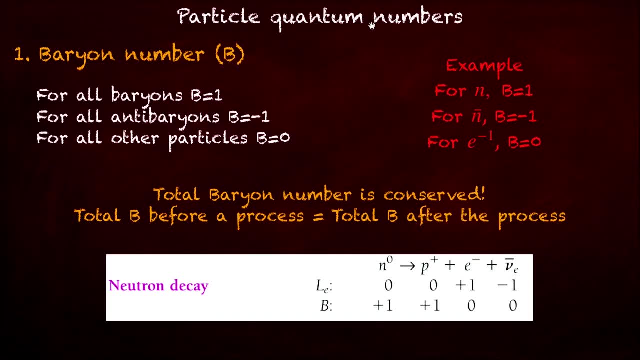 and the decay process in the order can do, we can. so we can get introduced a particle quantum number. so not you're right, but I can love the move. the type will apply to the number particle quantum number on a political level. first one is a very own number. video number of soaja between electronic team and. 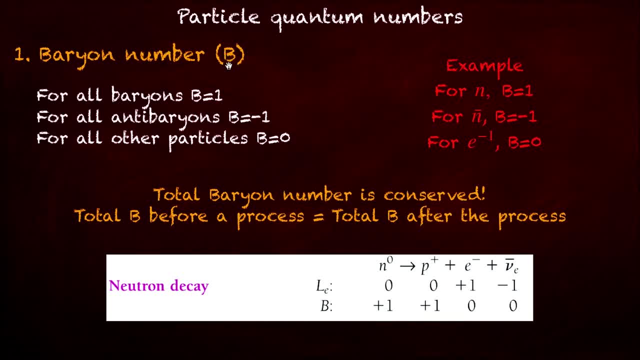 are available. number on the dish gonna look. so all the billions have a video. number is equal to 1.. In the baryon category there are nucleons and hyperons. In that category all the particles are assigned a number. That number is b equal to 1, plus 1.. Now all the 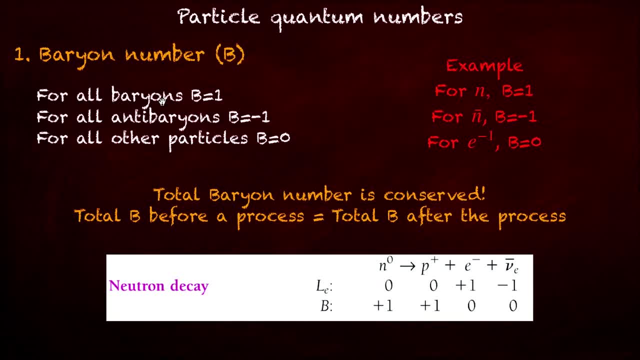 anti-baryons. that is, each particle has an anti-particle. If it is a neutron, its anti-particle is anti-neutron, as well as the anti-particle of proton is anti-proton. So for each baryon, 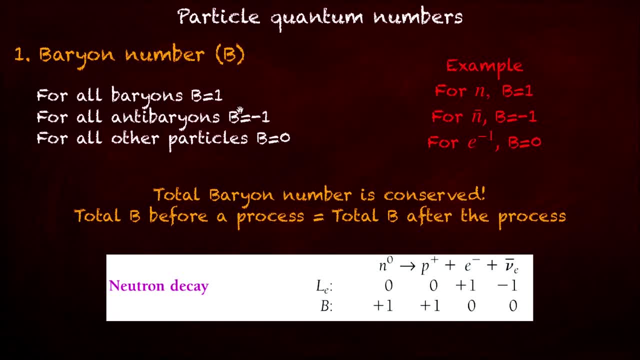 like this: the anti-particle has a baryon number which is the opposite of 1, plus 1 is the opposite of 1, that is minus 1.. Now all the particles other than the baryon and 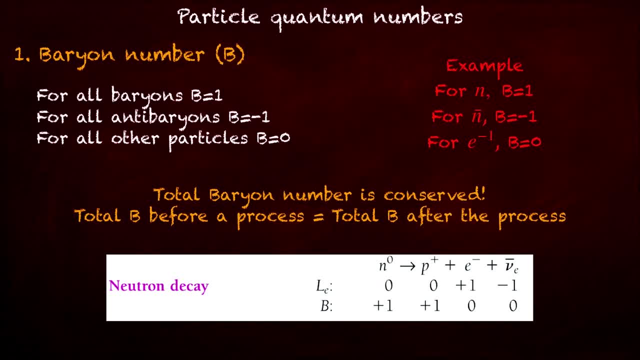 the anti-particle of baryon have a baryon number of 0.. For example, here the baryon number of neutron is 1.. The baryon number of electron is 0.. What is the importance of this baryon number is that 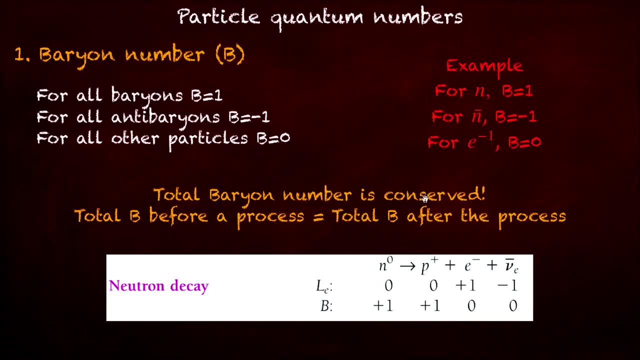 the total baryon number is considered. That is, the total baryon number before a process or decay is equal to total baryon number before a process or decay And the total baryon number after the process also means that before a process, of decay is of any value. 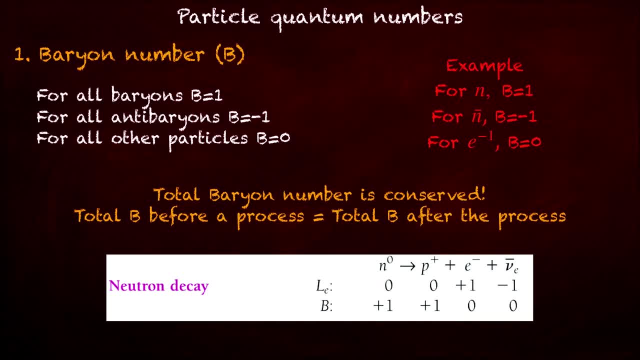 the total baryon number, before that occurs, becomes equal to the value of v of baryons of all the foreign particles that can be found in the baryon number. So if the total baryon number is equal to the value of the entire binion in the baryon, where the total baryon 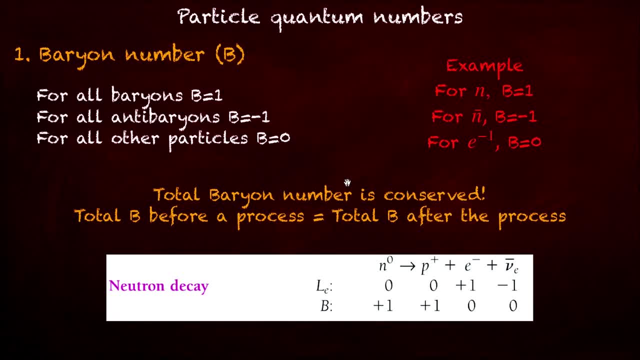 number is equal to the weight of the baryons. In that case the value of the entire baryon, It is the same. That is why we say that the total baryon number is conserved. I have given an example. I have given a neutron decay reaction. 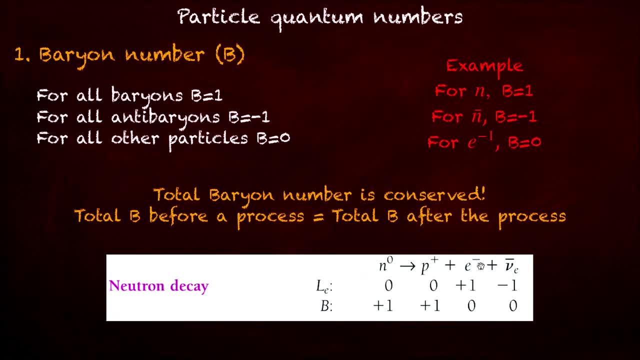 Here a neutron becomes a proton electron and an antineutrino an antiparticle of an electron neutrino. In this process, look at the baryons. Neutron is a baryon, So its baryon number is plus 1.. 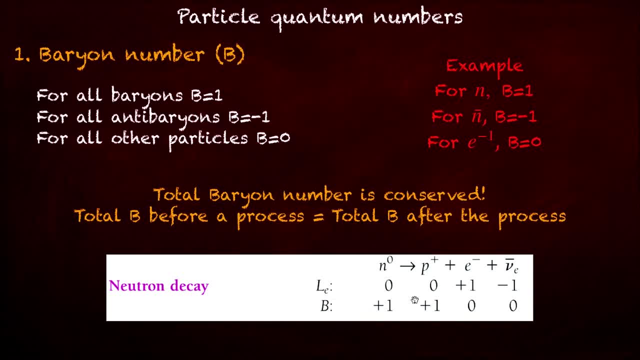 Look at the line at the bottom. If you look at this line, you can see that the baryon number is conserved. Since the neutron is a baryon, its baryon number is plus 1.. The proton is also baryon number 1.. The electron is not a baryon, so its baryon number is 0. 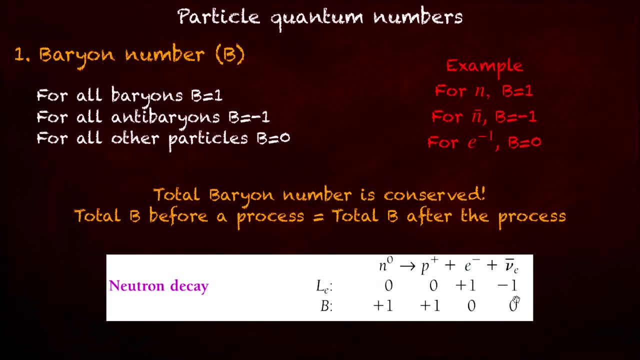 The antineutrino is not a baryon, so its baryon number is 0.. You can see that Before the reaction there is only one particle and its baryon number is 1.. After the reaction, after this decay process, there are three particles and all these baryon numbers will be added up to give plus 1.. 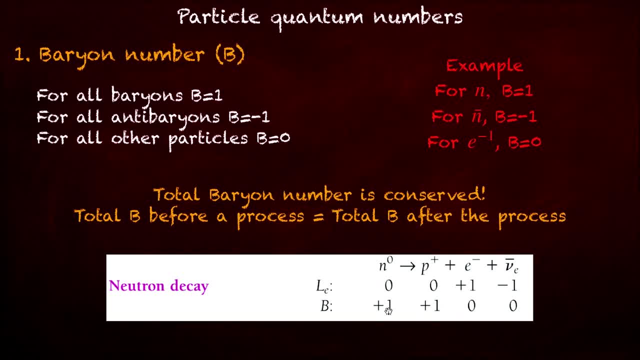 Which is equal to the baryon number before the process. So the baryon number before the reaction and the baryon number after the reaction will be the same. So the baryon number is conserved in all processes. 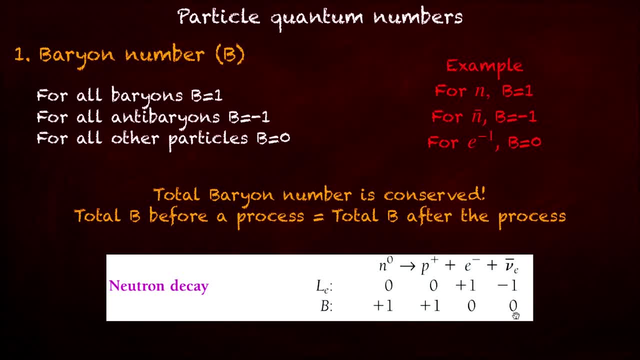 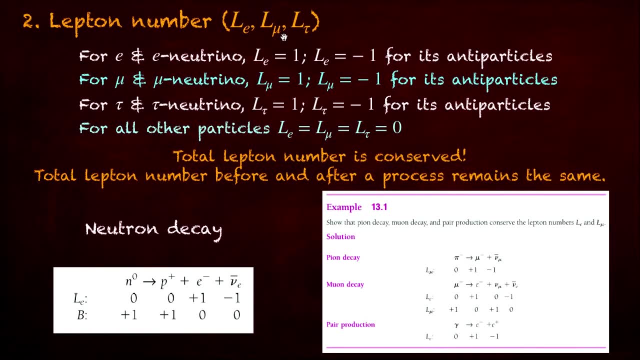 The baryon number is conserved in all types of processes. Now the next one is the lepton number. As I said earlier, the baryon number is a lepton number, but there are three lepton numbers, That is, electron lepton number, muon lepton number and tau lepton number. 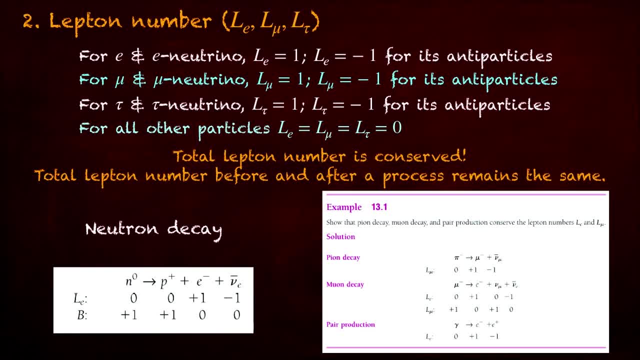 Okay, As I said earlier, in the baryon case, electron lepton number is equal to electron and electron neutrino. So electron lepton number is equal to plus 1.. Similarly, the antiparticle of these two, that is the antiparticle of electron, is positron. 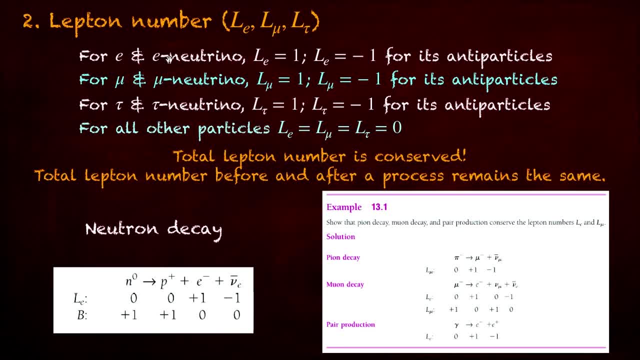 So positron and lepton number is equal to minus 1.. Similarly, lepton number is equal to antineutrino and electron neutrino is equal to minus 1.. Okay For all other particles: electron and electron neutrino and the antiparticle of these two. 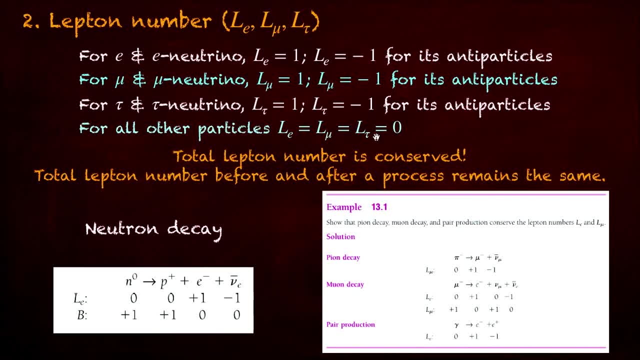 for all other particles, electron lepton number is equal to zero. Okay, That is the bottom line. L is equal to zero for all other particles. Okay Now similarly, muon and muon neutrino are equal to plus 1 and antiparticles are equal to minus 1.. 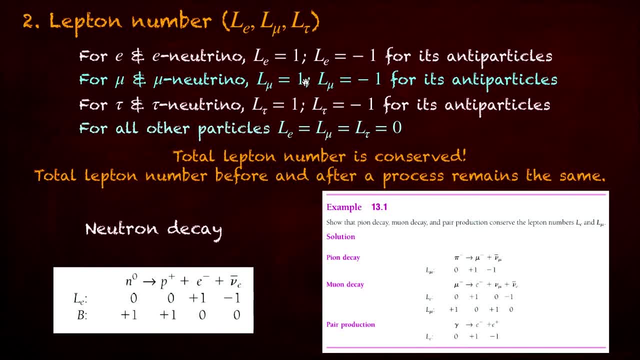 Similarly, electron and electron neutrino are equal to minus 1 and antiparticles are equal to minus 1 and 2.. They are not present in muon- neutrino and its antiparticles, So element electron has acting number of muon and its antiparticles is 0. 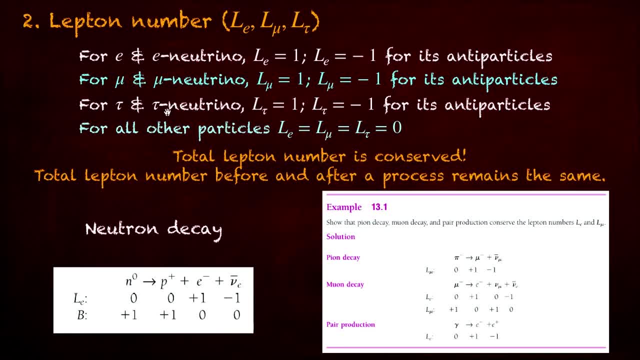 Because it is not coming into muon-neutrino and antiv. cooperate with caracter zero at the wall, to name it. Oh, left on number. so the game down in the particle. at all neutral, no other corner here, and the particle day, and the particle in the. 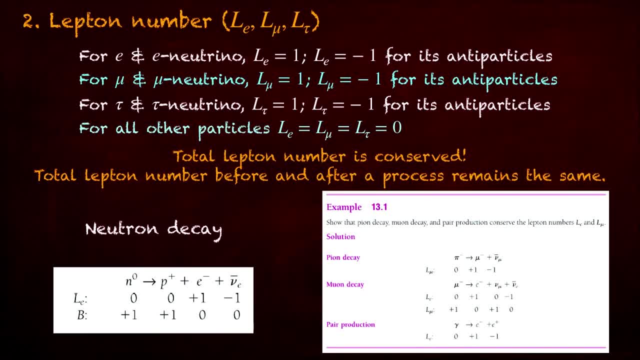 case alone. and there again now, left on number one barricade present article in a towel on the water towel, neutrino key. left on number one plus one. I reckon I didn't learn the nandy particle left on number minus one. okay, Mattella particle number zero. I know they don't number conservation. 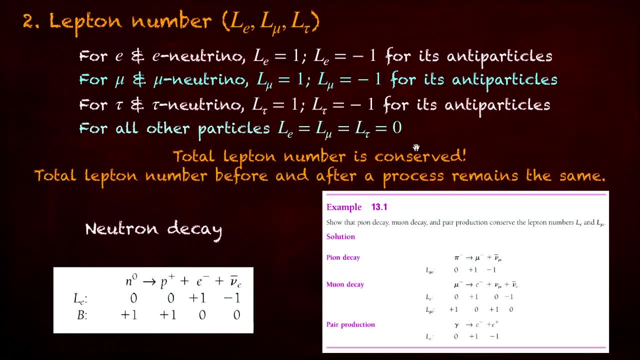 part of the total left on number is concerned in all process, in all process. another one right I'm similar to statement on the left on number. second, sold out in a lot of numbers: electron left on number and the new left on number and the towel up to. 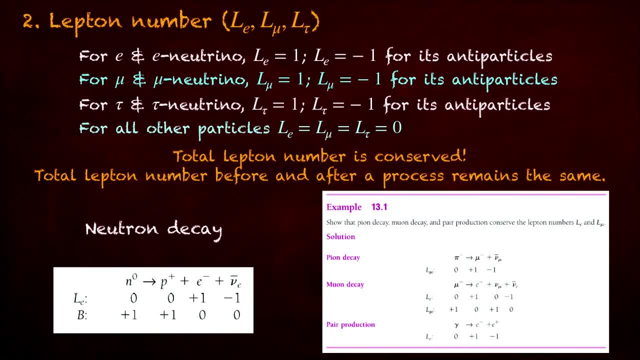 number under the alarm in a process, in a concerted. okay, now they are third number, let it the new tone, the DK process on the little of the left on number concern. so I'm going to look up, okay, neutral a little bit, you know. left on number zero, I did okay. 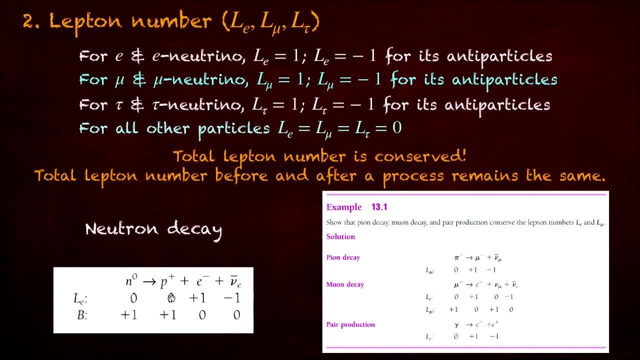 electron left on number on the cons, considering: okay, because if the electron on electron, electron neutrino on a little much a new one on you know it's now particle showing the tone down to the one Sir. electron left on number, okay. electron left on number hockey, the products or 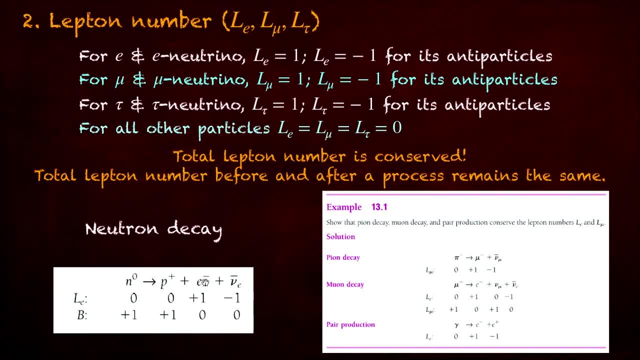 durumbrow down, you knowсол topping of a real another over there. electron up to a number of zero, like 1985. electron left on number, It was one. and The Do-감 neutral, Anti electron neutral, dceptathlon. tell us to learn something better. 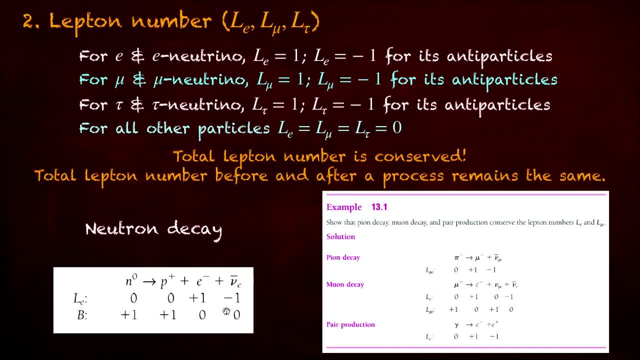 from Brian super UX and the whole thing. Они want you to know the end. I can't Пред viscosify digitalsim entrepreneurs. You can't predict what happening on there. from this value of theił, the electron number will be minus 1.. Electroneutrino will be plus 1 and the antiparticle will be minus 1.. 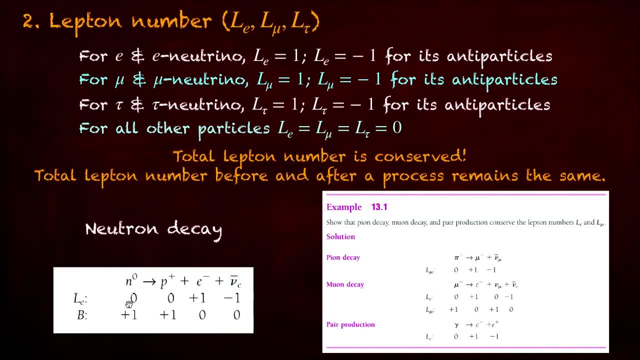 Now, before the reaction, the electron lepto number will be 0.. After the reaction, it will be 0 plus plus 1 plus minus 1.. After adding all these, it will be 0.. Now this reaction is indicated that the electron number is considered in the neutron decay process. 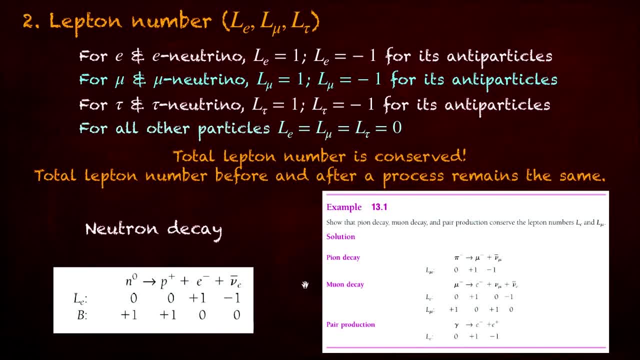 Now I have given other examples here. This is an example given in the text I have given: the decay of pion. The antiparticle of pion is pi minus mu minus plus mu neutron. It has changed to an antiparticle. 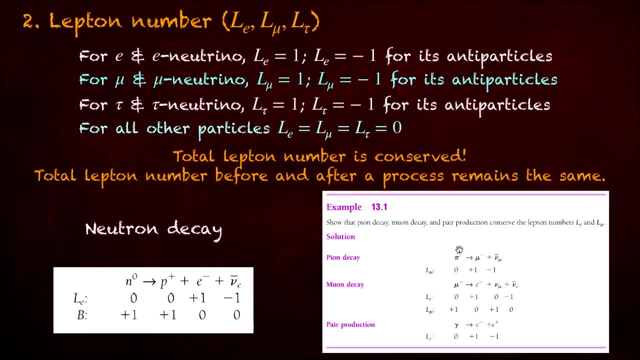 Now, if we take the mu lepto number here, the pion is meson, So its mu lepto number will be 0. So mu 1, lepto number plus 1, and its antineutron will be minus 1.. 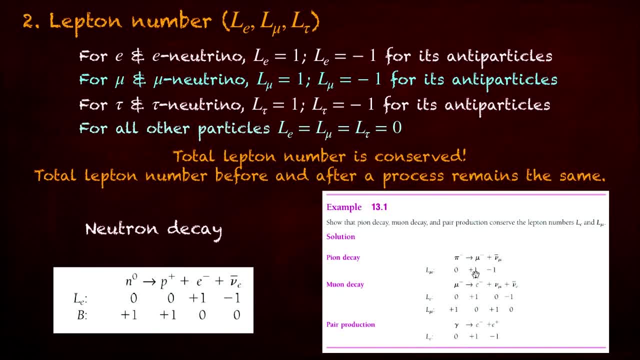 So before the reaction it will be 0.. After the reaction it will be plus 1 plus minus 1.. So mu lepto number will be conserved. So mu 1 decayed. So mu minus decayed to 1 lepto number. 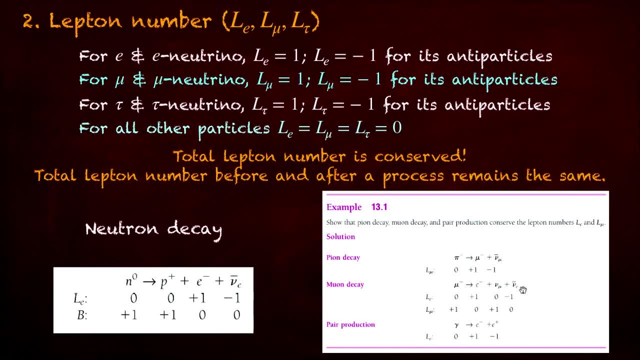 So mu lepto number is conserved. So mu of this lepto will be раздел in 2, Levi is not visible and mu neutrinon will be left in black. So the electron number of each lepto will beSelected then. 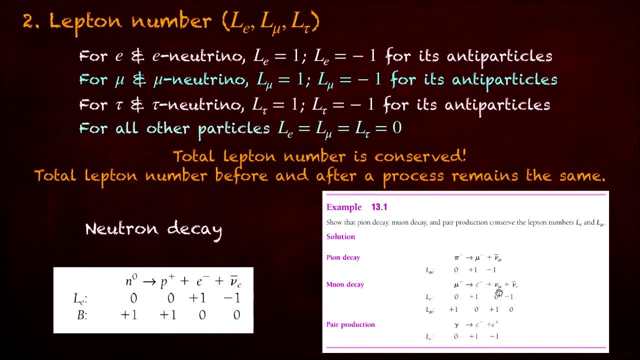 So ref六 y i and mu neutrinon will be the traditional Cardinal. A lepto goes to zero and a Mus B omega goes to zero. So says mu neutrinon and the electron lepto number. here This will be neutral. 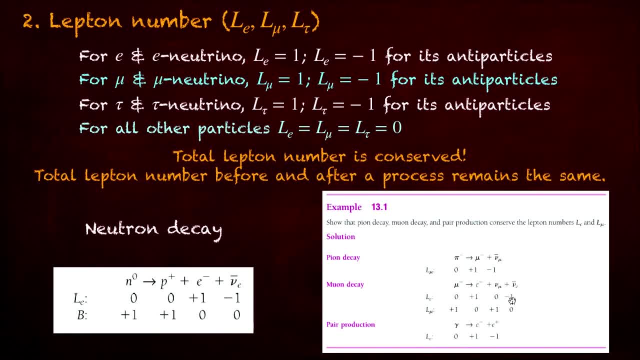 So this is an function of the mu neutron, This is neutral electron electron-neutrino, And this is the mu direction-ley создane. Before the reaction: electron-leptone number is 0.. After the reaction: plus 1,, plus 0,, plus minus 1.. That too will be 0. 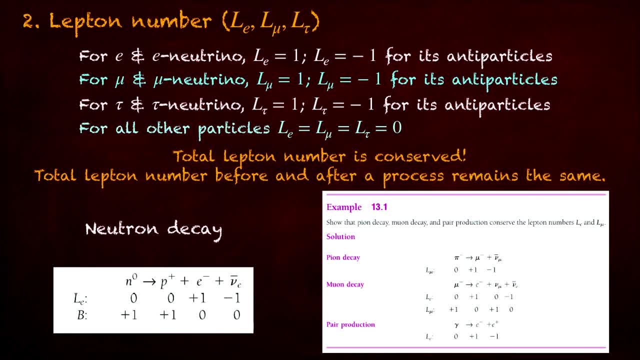 That is a process of conserving electron number In the same reaction. let us take mu electron number. When we take mu electron number, mu minus particle's electron number will be plus 1.. Electron: mu electron number will be 0.. For mu neutron number, mu electron number will be plus 1.. For anti-electron neutron number, mu electron number will be 0.. 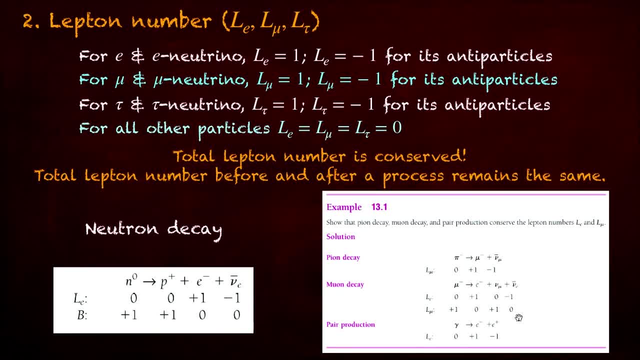 Before the reaction plus 1.. After the reaction plus 1.. Mu: electron number is conserving. Now the process of pair production. The process of pair production is when a photon comes and becomes a electron and positron pair. The process of pair production is when a photon comes and becomes an electron and positron pair. 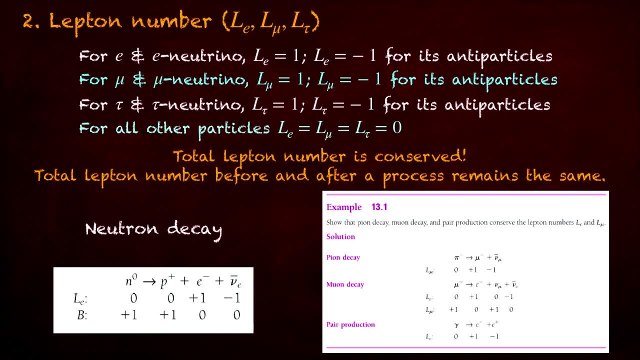 This is the process of heavy nucleus. In the presence of a heavy nucleus, a photon. Before the reaction: 0.. After the reaction: 1, plus 1, plus minus 1.. That is also 0.. 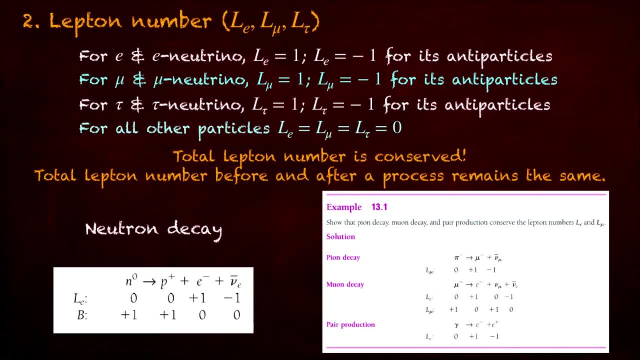 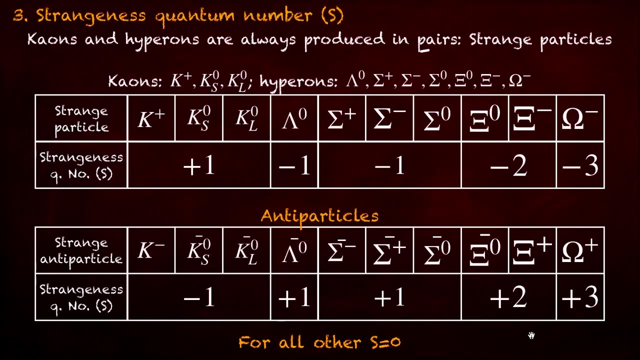 So electron-leptone number is conserved during pair production. Now we move on to strangeness quantum number, which is denoted by S. Before telling strangeness quantum number, what is a strange particle? A strange particle is a k-mason of K plus Ks0 and Kl0.. 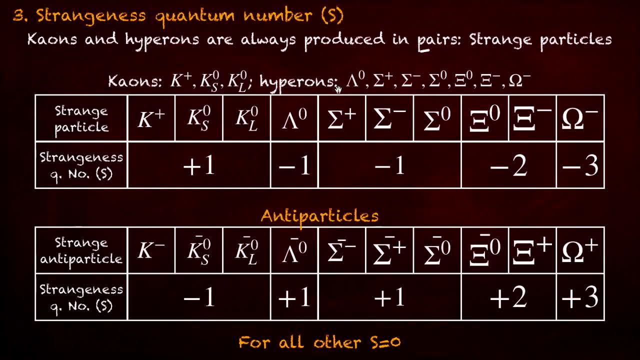 Also a hyperons of K plus, Ks0 and Kl0.. Hyperons are the particles which are transferred from the nucleons to the baryons, In that lambda0, sigma plus, sigma minus, sigma0, and sigma minus are the hyperons. 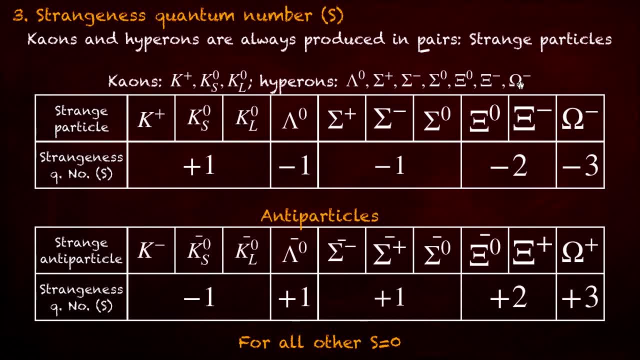 The other particle is the hyperons. The particles in these two categories are always produced in pairs. When a reaction takes place, they are always created in pairs. If a k-mason is created, there is another k-mason beyond that. If a hyperons is created, it is not created as one hyperon, but as a pair. 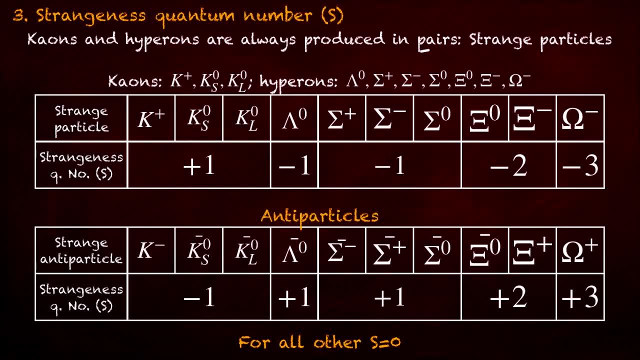 There is a strange behavior like this. Let us see For that. a quantum number called strangeness quantum number is assigned. The name of this particle is strange particle. The strangeness quantum number of this strange particle is given in this table. You have to understand this. 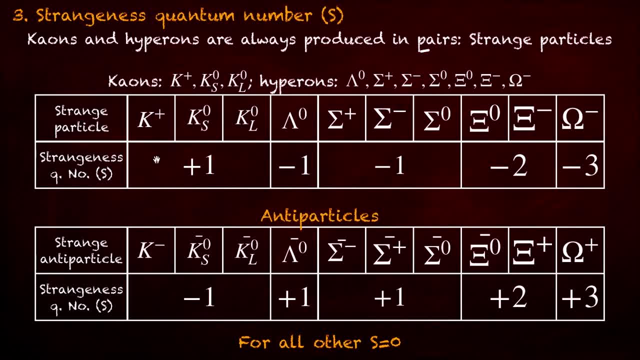 So strange particle. The strangeness quantum number of k-masons is plus 1.. So lambda0 is minus 1.. For sigma particles, sigma plus is sigma minus. The strangeness quantum number of sigma 0 is minus 1.. 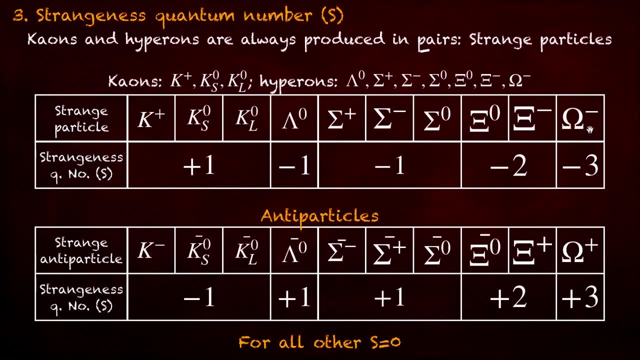 For xi0 and xi minus, the strangeness quantum number is minus 2.. For omega minus it is minus 3.. Now if you see here, you can see that the strangeness quantum number of the strange particle is given in the anti-particle. 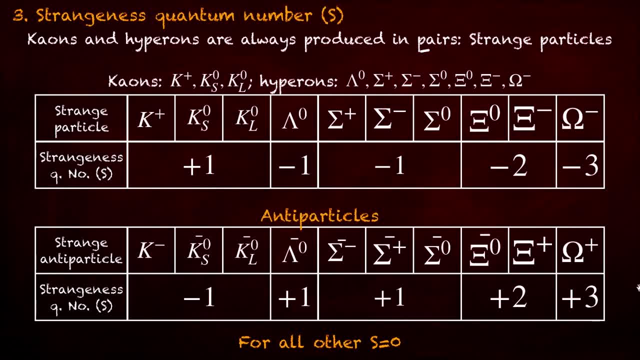 The strangeness: quantum number of the anti-particle is given in the table below. What is there here? It is directly opposite. It is here For the k-masons. the anti-particle of k-masons is k plus and k minus. 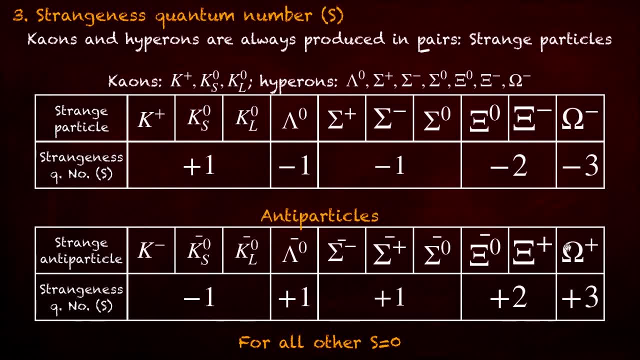 These two must not change. For the rest there cannot be a confusion, that the strangeness quantum number of all the three must not change. For the confusion that arises, the surprise of k plus and the strangeness quantum number of xi minus must also be given in the canons here. 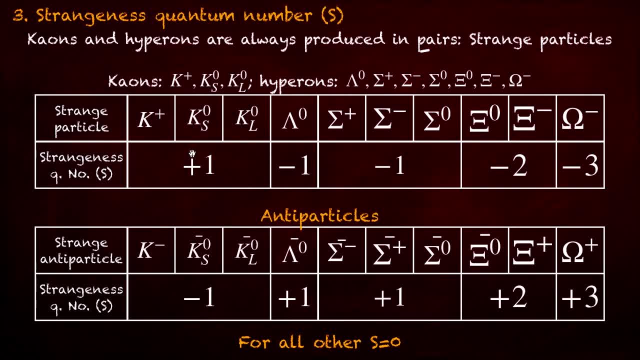 k plus is the anti-particle of k minus. The protizing power of anti-particle must be minus 1.. The strangeness: quantum number of the three particles in front of it is plus 1. and the anti-particle K minus. Ks0 bar, KL0 bar and the 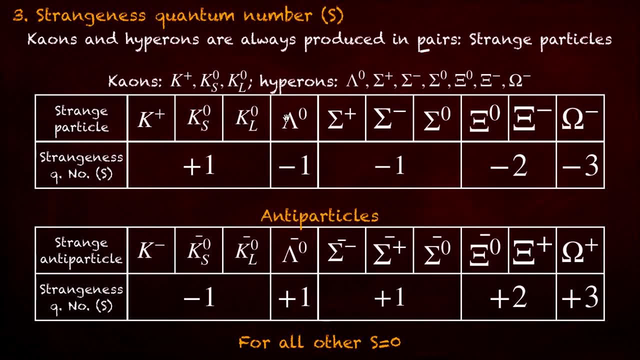 strangeness: counter number minus one. lambda zero minus one item and the anti-particle lambda zero bar plus one on a strangeness counter number and the world: a sigma minus a sigma plus sigma plus, sigma minus sigma zero. so a moment, strange respond: a number one minus one item from Sigma plus in the anti-particle. 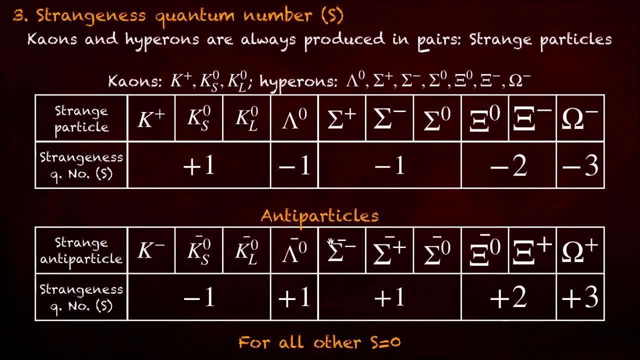 another charge, Murray, Sigma minus. I have a part in a bar, the Sigma minus bar, on a Sigma plus in the anti-particle, Sigma minus in the anti-particle and on Sigma plus bar on, okay, Sigma zero and anti-particle Sigma zero bar. so then the 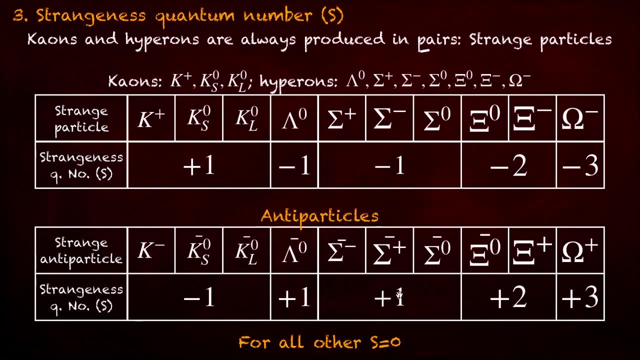 he move the part anti-particle name: strange, respond a number plus one on. okay, I've got a side by zero, sign, sign minus other than that stranger, stronger number, minus to arrow and anti-particle in size, euro you side plus the bar, vanilla bar, a lot of the K plus in the anti-particle here when I say: 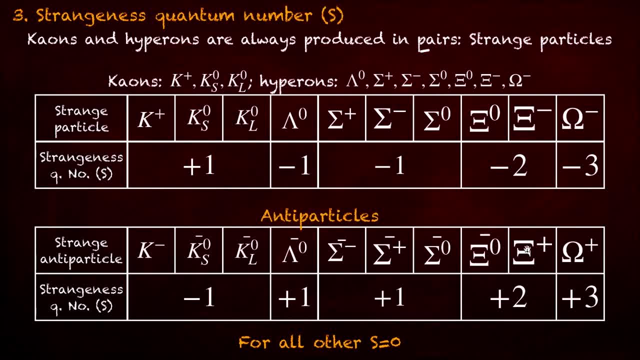 minus an anti-particle in the barrel in there. okay, I'm size 0 bar. no, I plus in the strange respond a number plus two. okay, now the particle Omega minus is covering and strength-less corner number minus three and it's antiparticle. Omega plus is having a strangeness conda number plus. 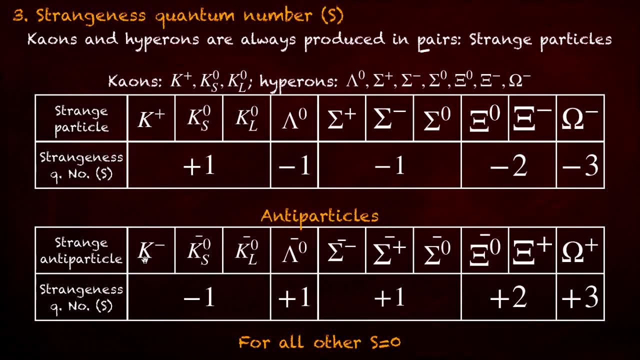 three. okay, now we will put it in the antiparticle system, K minus psi plus Omega plus, between particles in there, particles in a antiparticle. I tell everyone the summit of the bar and in the top of the bar, we don't know. okay, I'm gonna program and the particle, the charge, a bottom and in the near opposite. 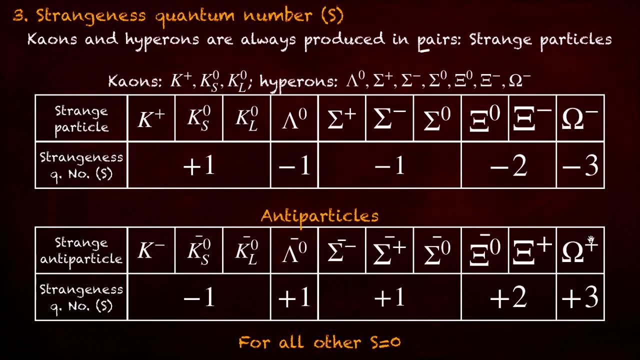 charge which it on and the antiparticle. so to pick. okay, now L last race particle, now the strangeness conda number and the antiparticles. strangeness, conda number. and okay, either kodada, illa, matilla particles, strange particles, a lot of aquila particles. 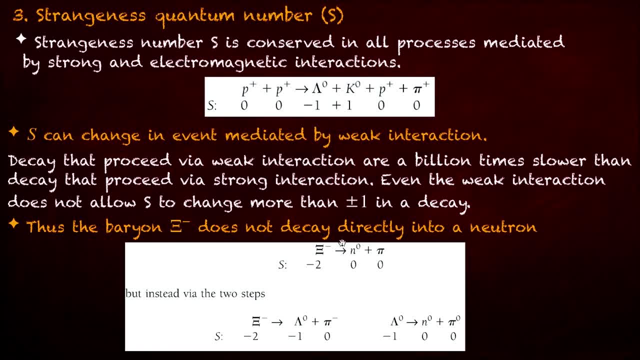 now number, the very own thing left on the game number. conservation of the electron number. conservation, Allah, permanent, the very own number of electron number in the process in concern. okay, actually with a stringiness component, but considering the summit, the strangeness. quantum number in the process in concern. Allah, okay, it is. 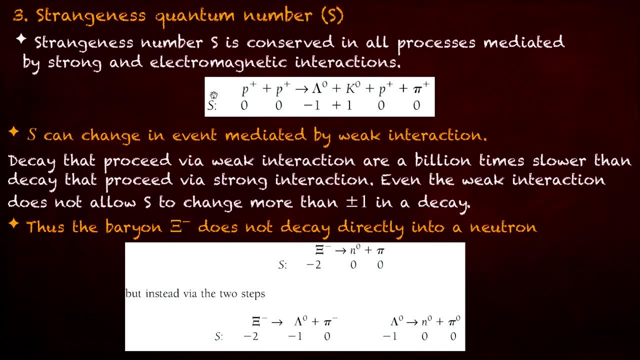 concerned on with the in all processes mediated by strong and electromagnetic interaction: strong interaction of the wall, a electromagnetic interaction mediating the process in matram on a stringiness, quantum number, and so on. so, other than the example, on a little particular, and the protons collided a. 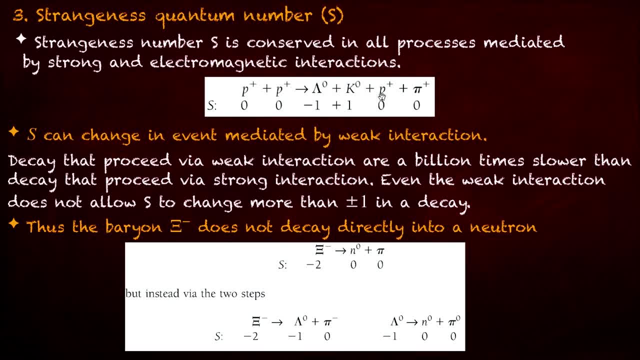 bit about the particles on a lambda 0 K, 0 and sub proton and a pi plus particle he process in the mother proton decoration, either the strong force mediating the process on a, for you case the stringiness quantum number concert on. on check here it wasn't a shaped an example, but the wrong way, as shown by uh. 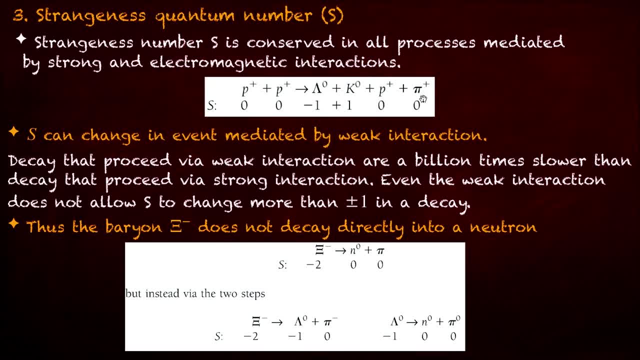 here for not Nick. go on Co. Additionally on a number of zero, three preferences, as you can see. you can see, okay, each of these are the three following: so we talked about only 1,, 0 andminus 1.. However,1 andminus 1 is not strange numbers, It is 0.. K.0.. got to forget that number of 1,. So at second calculation, to shape it in a certain way, this is 0, 1. outside it is all 2, большой area. you would not be able to understand that the reaction is positive root formulae. therefore it is not strange number. The first one is 2,. also, if you homogenization is thisstaggiantem. 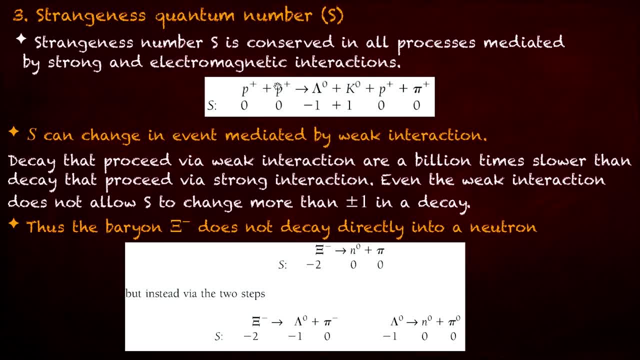 process. this is a process mediated by strong force, and here the strangeness quantum number before the reaction and after the reaction is the same. okay, now we are going to observe that the strangeness quantum number is conserved only in the process of strong interaction and electromagnetic interaction. 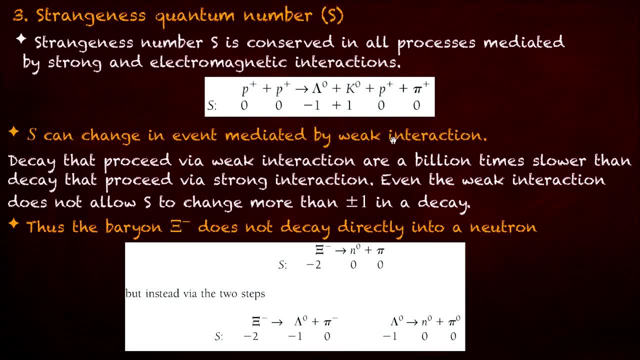 if the weak interaction is mediated, then the strangeness: quantum number is not conserved. even if it is not conserved, there is a limitation. even the weak interaction is not conserved. the weak interaction does not allow s to change more than plus or minus one in a decay. 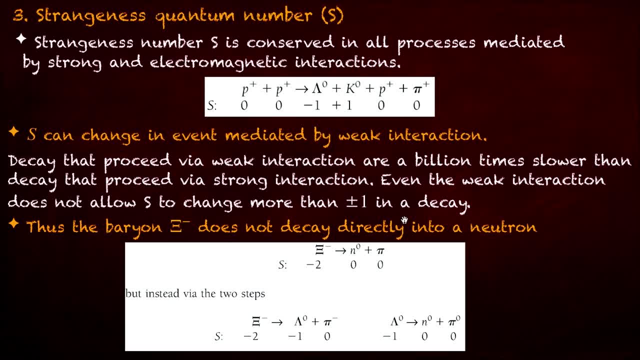 that is the difference in the strangeness quantum number. the difference in the strangeness quantum number before the reaction and after the reaction can not be any number. the difference in the strangeness quantum number can be plus or minus one. for example, let us look at the decay of a baryon. 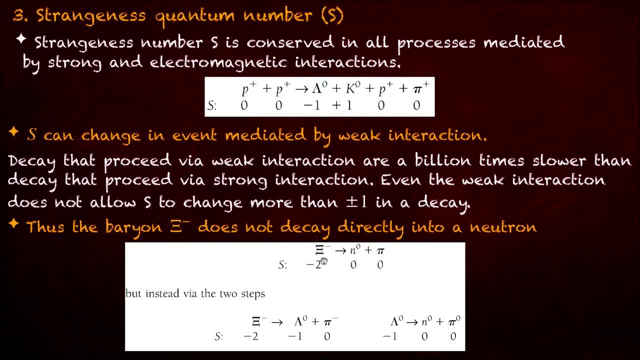 let us look at the decay of a baryon. according to this decay, neutrons and pi ions change. now here the strangeness quantum number. the strangeness quantum number of psi minus is minus two. neutrons is zero and pi is zero. so, before the reaction, the strangeness quantum number is minus two. 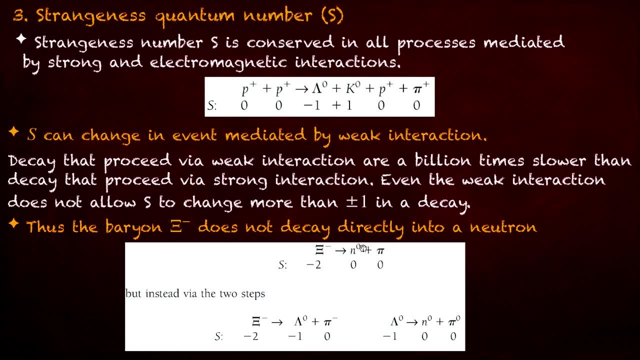 after the reaction is zero. so the strangeness quantum number after the reaction is two units more. so this is the process of weak interaction mediated. so when this happens, this is the rule. this is the process of weak interaction mediated. so the strangeness quantum number is minus two units. 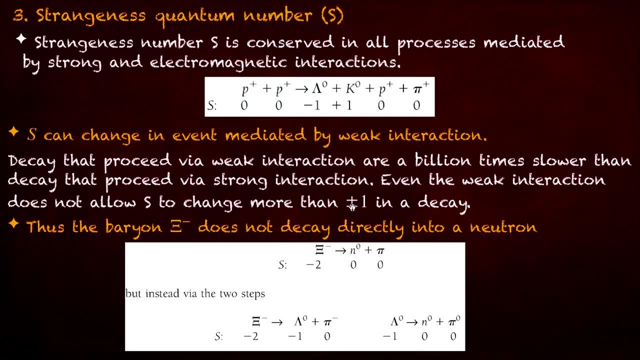 Strangeness: quantum number one unit should increase or decrease, but here you can see that two units have increased. Later, to explain this, when we investigated this reaction more, we understood one thing: This is a direct decay. The decay takes place in two steps. 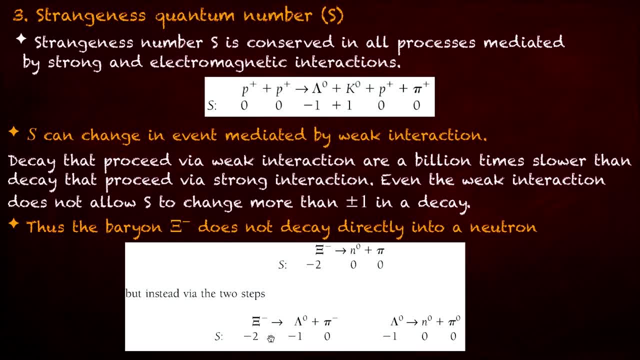 In the first step, psi minus changes from lambda 0 to pi minus. If we take the strangeless quantum number from here, it is minus 2 lambda 0 to minus 1 pi to 0. Here the strangeless quantum number increases by one unit. 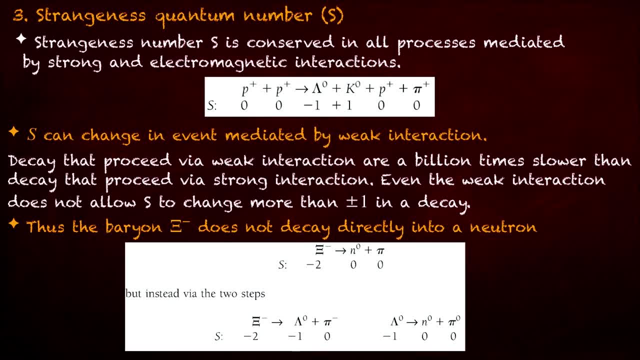 Minus 2 to minus 1.. Later this lambda 0 is decayed again and becomes neutron and pi Minus 1 to 0.. In this process, one unit increases Minus 1 to minus 1, becomes 0. 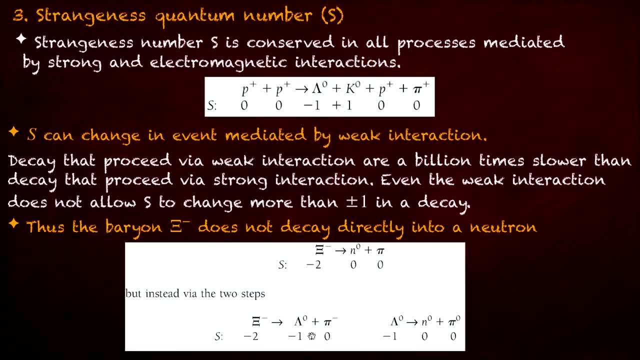 This decay changes to neutron and pi, So this is replaced and becomes neutron and pi. This is how this reaction is carried out. This reaction is not a direct reaction. It is an intermediate step. This is how it is carried out In any process. 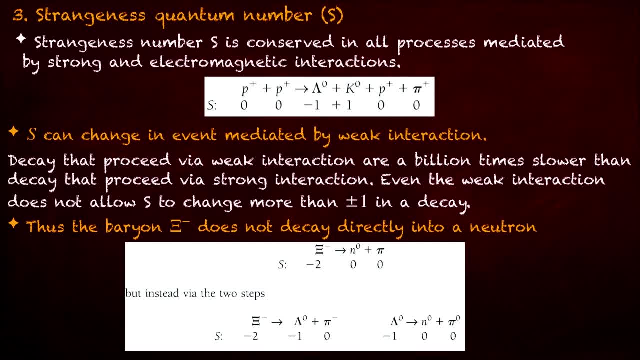 we can in any passive-interaction mediated process, we can not observe the strangeless quantum number. Even so, the difference between the strangeless quantum number is just a plus or minus 1 unit. In all processes, all processes which are mediated by strong and weak, 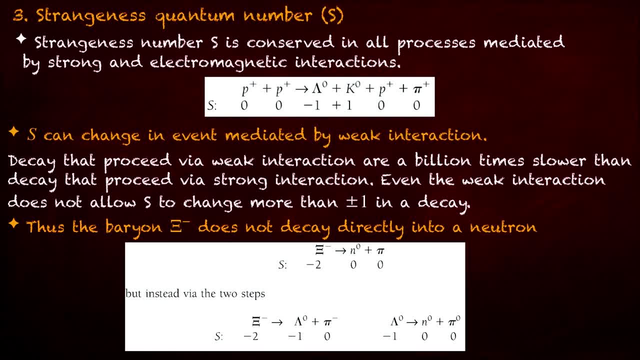 strong and electromagnetic interaction. the strangeless quantum number before the reaction and after the reaction should be considered. Here we have discussed three types of particle quantum numbers: One is the baryon number, the other is the lepton number and the third is the strangeness. 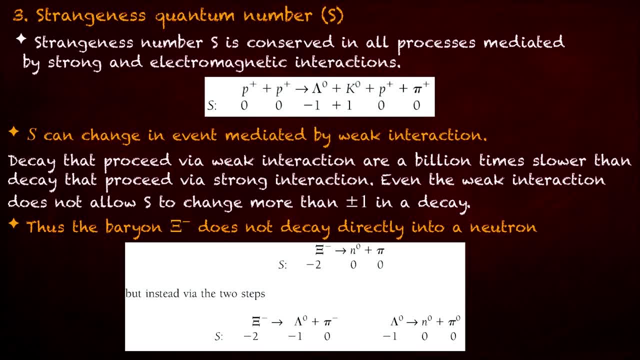 quantum number. Now, apart from these quantum numbers, there are other particle quantum numbers available, But for now we don't need to discuss other quantum numbers. According to your syllabus, we need to study these three quantum numbers, So we should. 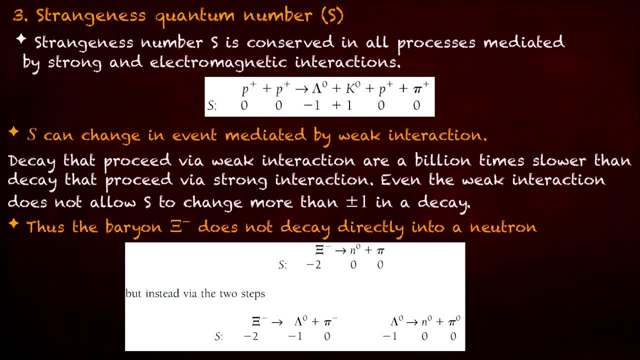 be thorough with these three quantum numbers and how to check the conservation of different quantum numbers. The baryon number and lepton number can be studied in all the processes which are conserved, But the strangeness, quantum number is not conserved in the process. 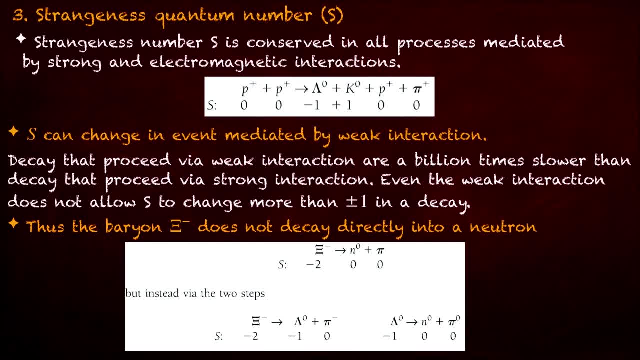 in which weak interactions are mediated. When we say that it is not conserved, there is a limitation. The strangeness: quantum number should be different in each unit in the processes which are mediated by weak interactions.